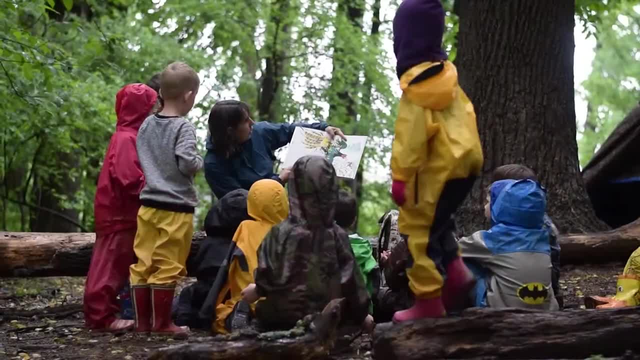 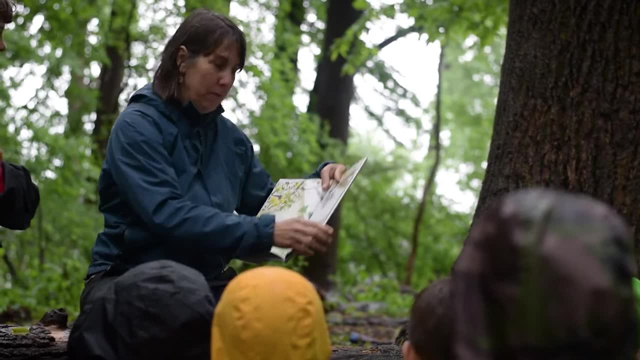 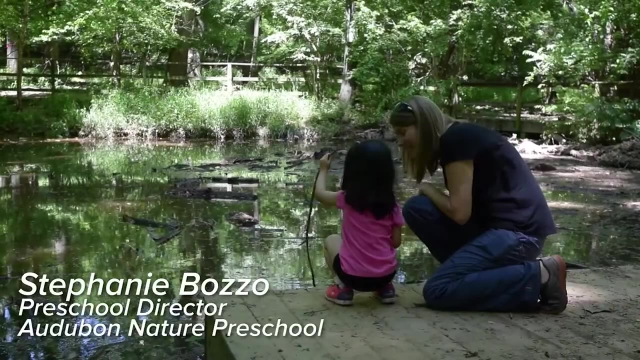 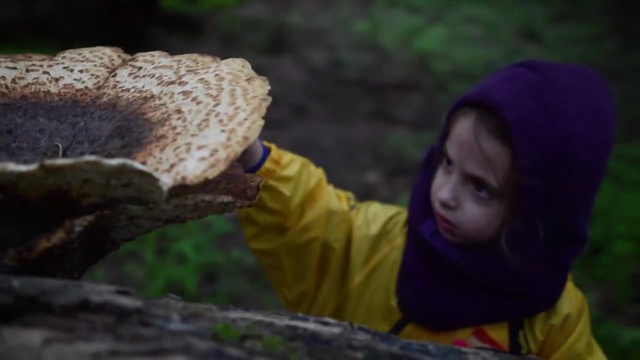 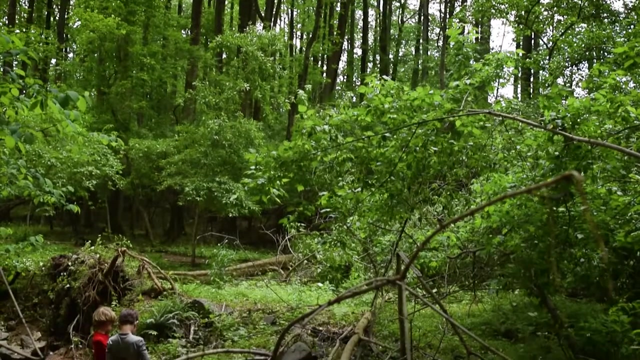 After that story time At the top of a hill you love so much, you'll never forget how it feels there. Why do we have a passion for connecting with nature? Because nature is the best teacher there is. Nature-based education emerges from children's interests and passions. 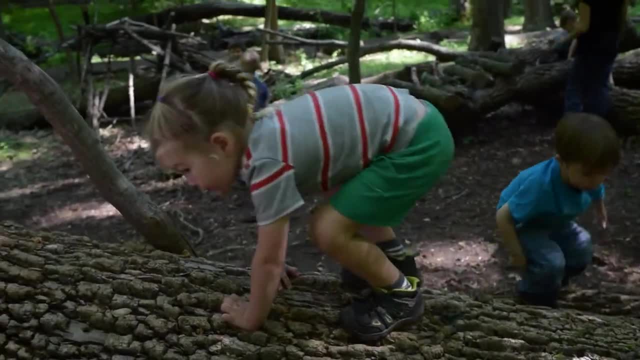 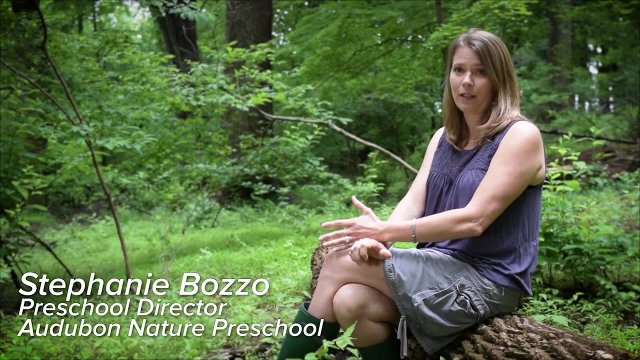 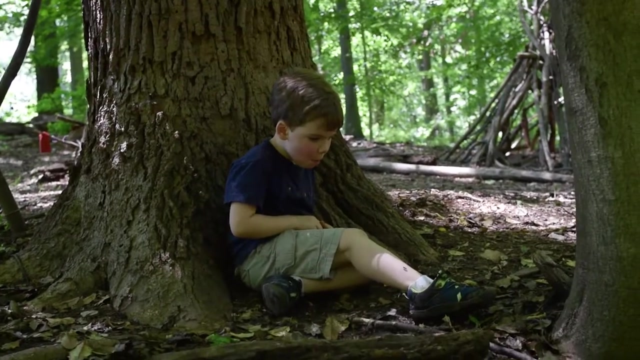 The growth that we see in each student is incredible And we really believe that's because nature is the great equalizer. There is something for everyone, Whether it's large gross motor skills of balancing on logs and jumping and leaping and chasing, Or if it's just quietly sitting and observing a caterpillar spin its chrysalis. 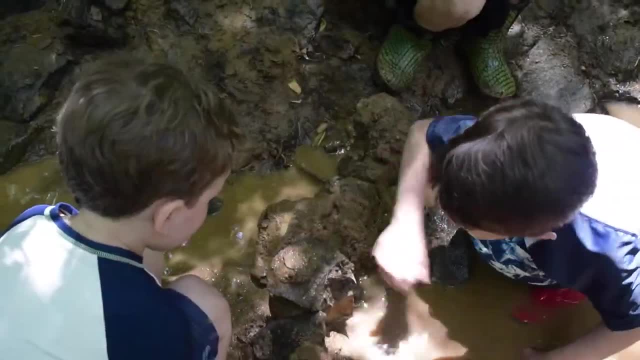 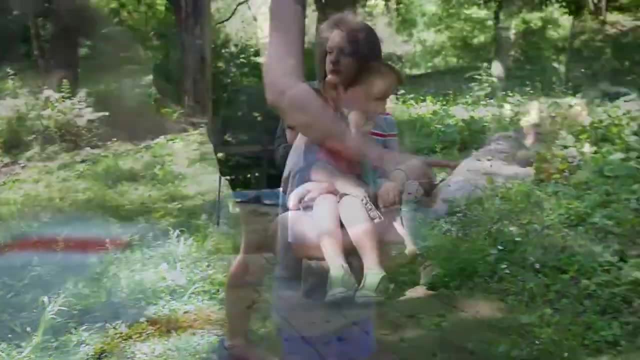 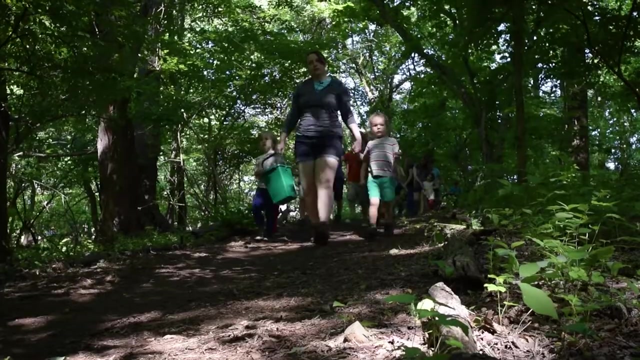 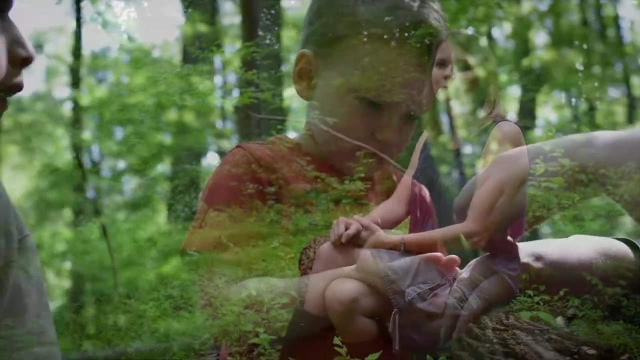 The joy that happens when children are directing their own learning is immeasurable. Children learn best in an environment where they feel safe and loved. Our teachers are experts at encouraging children and knowing exactly where each child's strength lies, So that when we take them out exploring in the woods, we really know where each child is physically, emotionally and mentally. 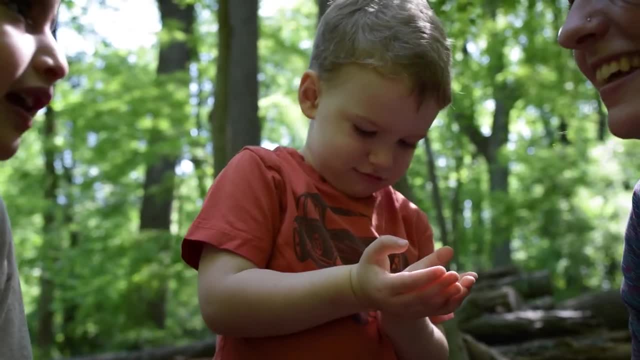 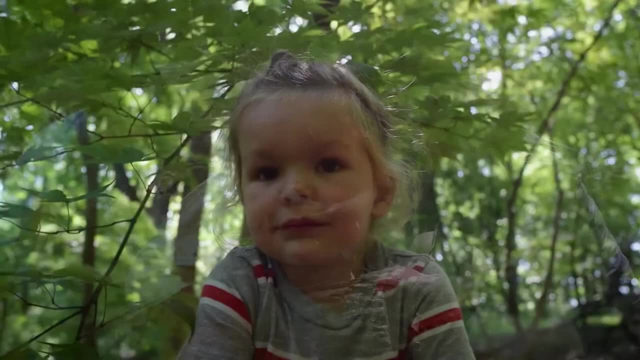 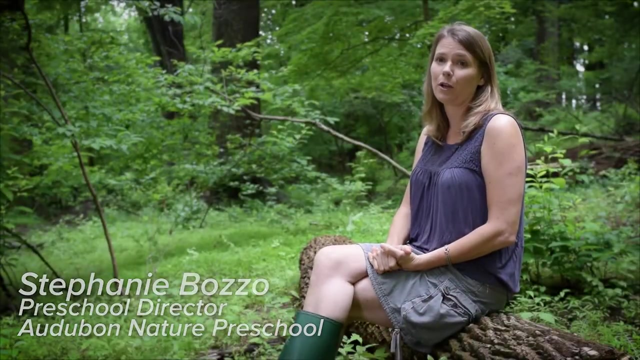 Children need to spend time in nature to fall in love with it, And having the children have those rich experiences in the same place, in nature, day after day, has been proven to provide a richer, more meaningful connection to the earth, Which is what will, in turn, help our children be the stewards of the world that we need for tomorrow. 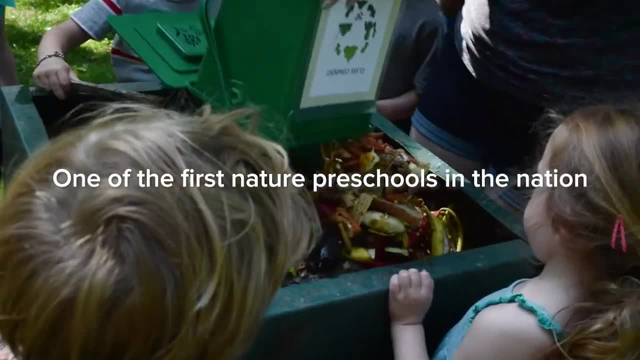 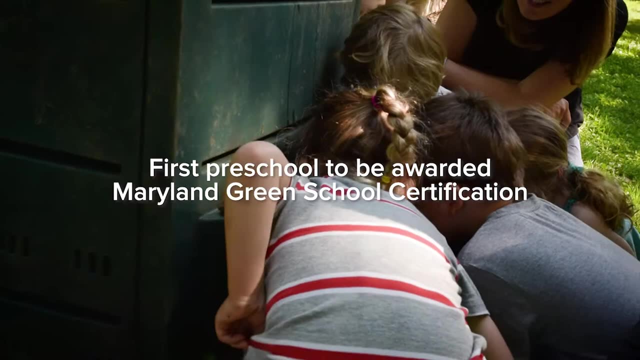 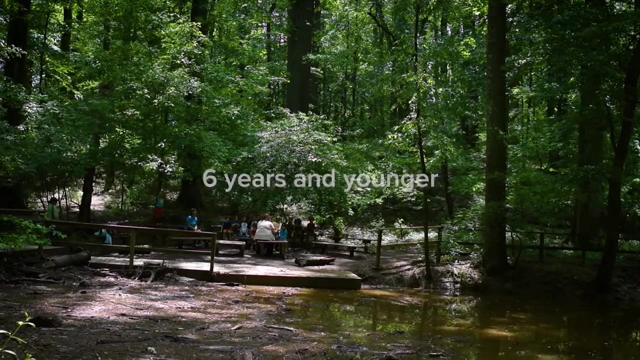 Here we go. Who do you think is going to be in here? Will we see Squirmy Wormy? Snack time, I guess for Squirmy Wormy. Good observation, Dad. She got completely muddy all over. Even her nose was full of mud. 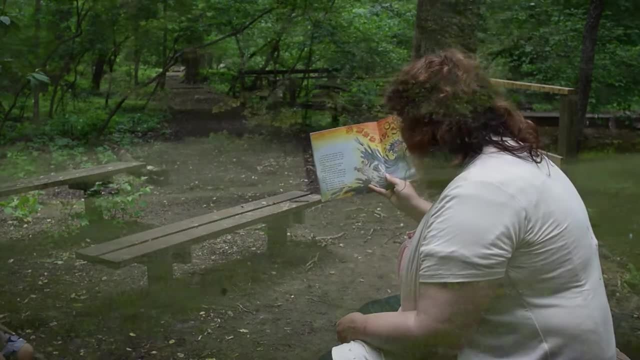 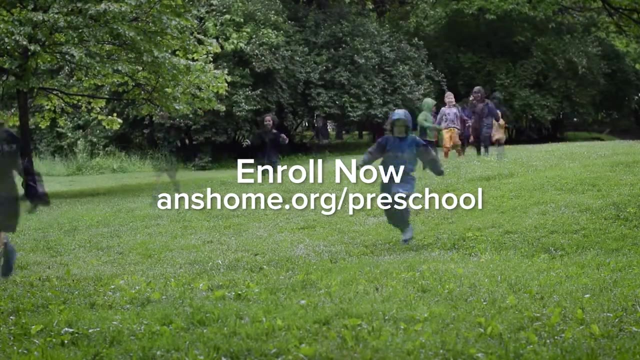 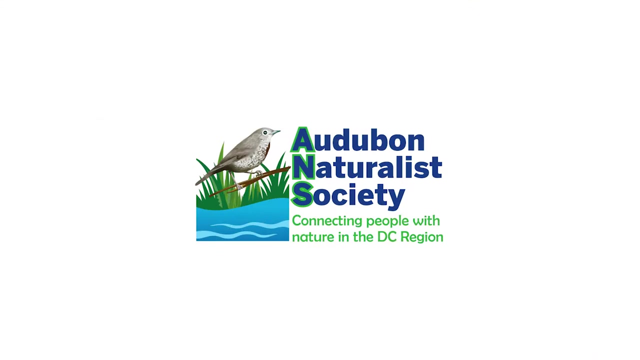 Jewel Ann ran inside yelling Mommy, Mommy. a mud puddle monster jumped on me. Jewel Ann, look She's a monster, She loves people.